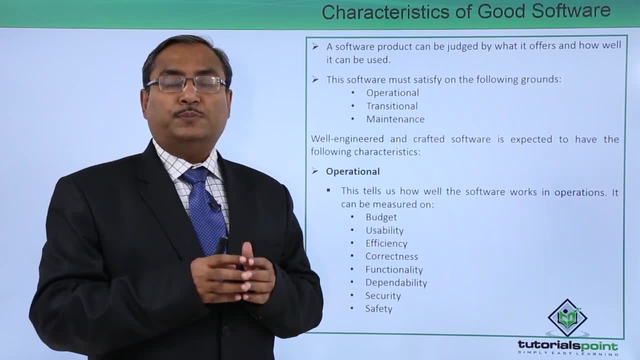 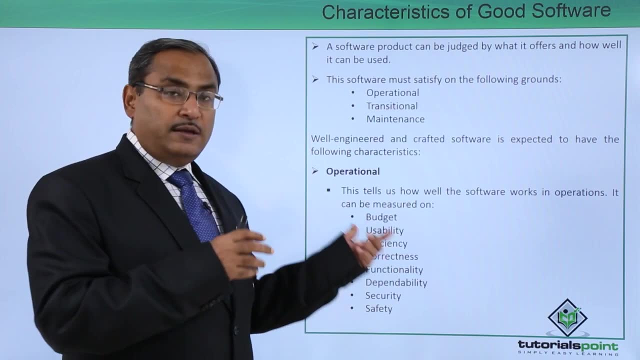 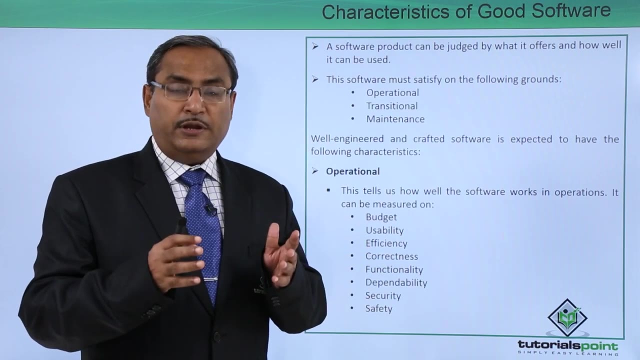 the budget. A software should have a good usability. Software should be efficient. It should be also very much secured. The safety of data is ensured. It is giving us the correct answers. correct results are getting obtained. It is efficient. That means it will give us the required result. 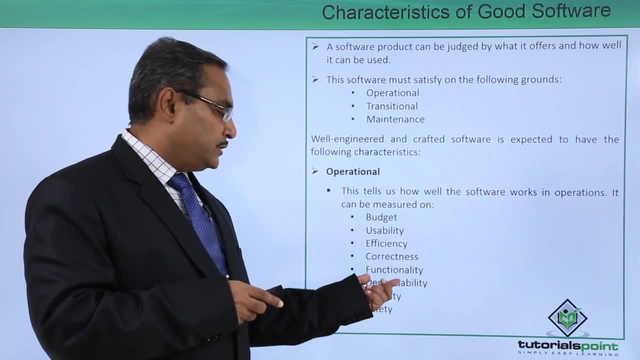 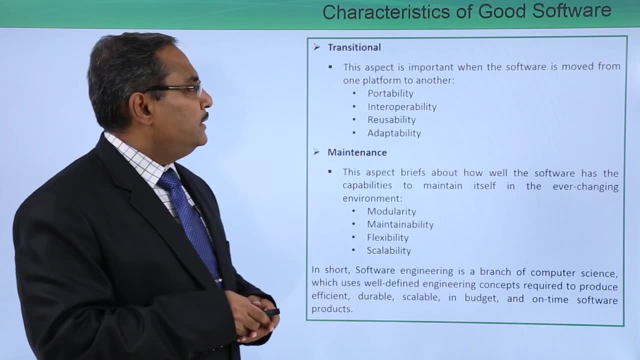 within the minimum optimum amount of time. The functionality, the dependability, so the efficiency needs to be there. These, all these are the features under this operational. So now, next, we are going for this transitional. This aspect is important When the software is moved from one. 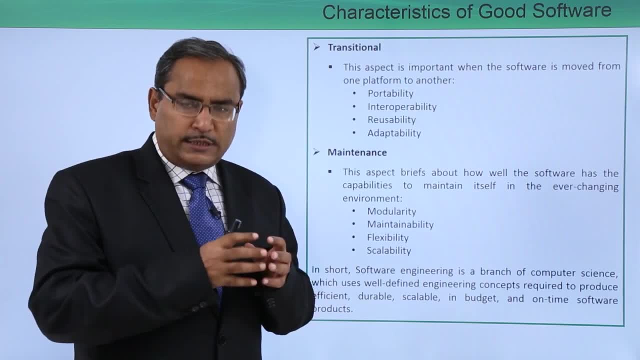 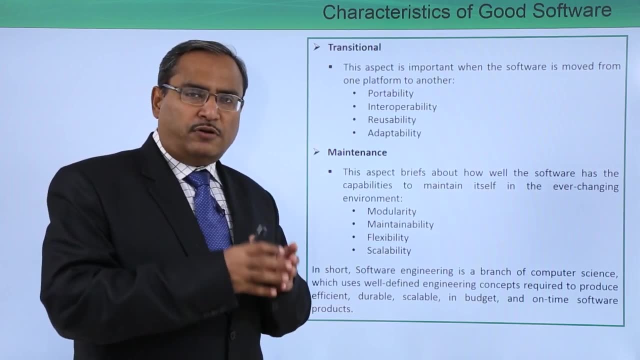 platform to another platform. So platform means operating system, the respective architecture of the system, Combined them. we usually call it as a platform. So whenever a particular softwares will be moved from one platform to another platform, then in the case the portability, the interoperability, the reusability and adaptability and C sag101. 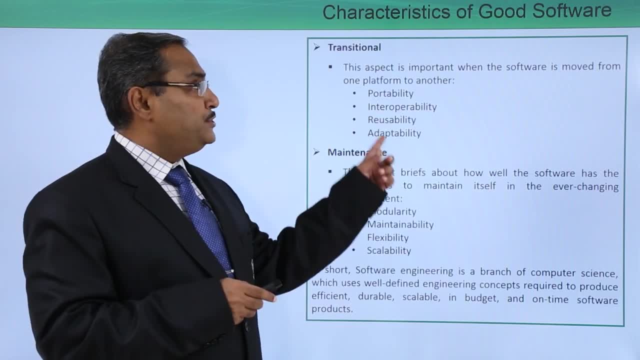 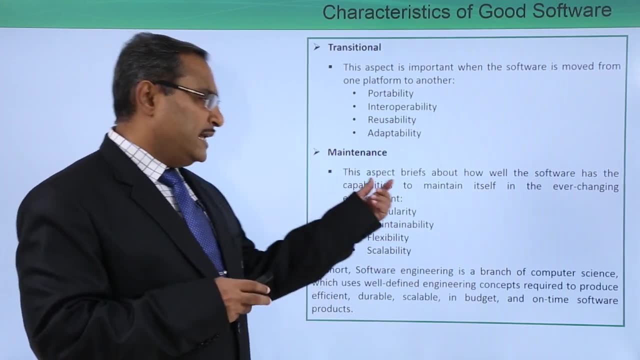 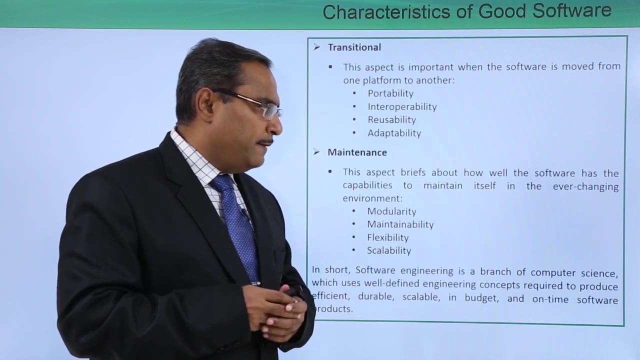 0 and adaptability are the main features under this transitional. Next aspect we are going to discuss is our maintenance. So this aspect briefs about how well the software has the capabilities to maintain itself in the ever changing environment. So that is our maintenance. 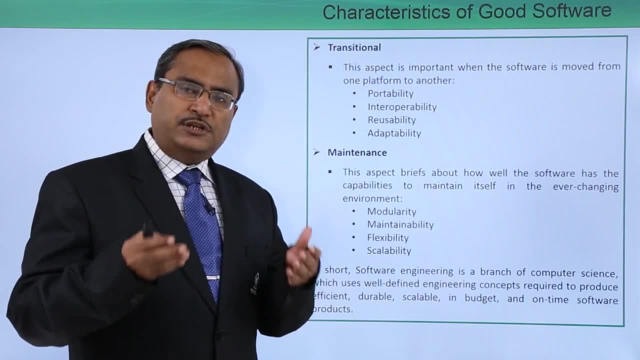 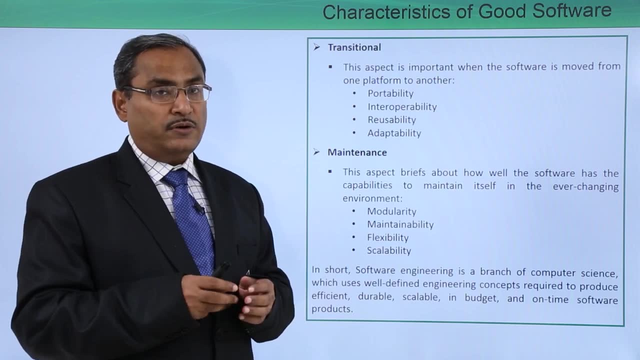 We know that whenever a software will be in operation, so multiple change requests will be coming. multiple changes are to be carried out on the software and that is falling in the part of the maintenance of the software, So how this maintenance can be fruitfully executed on the 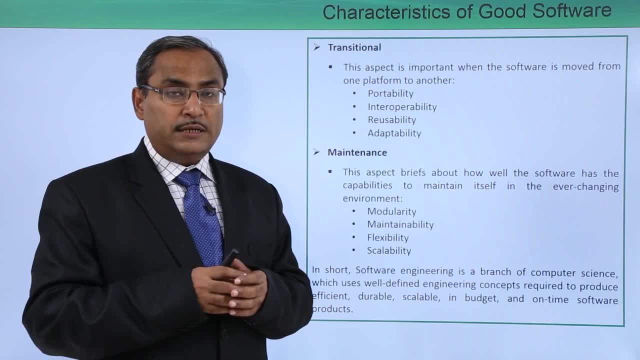 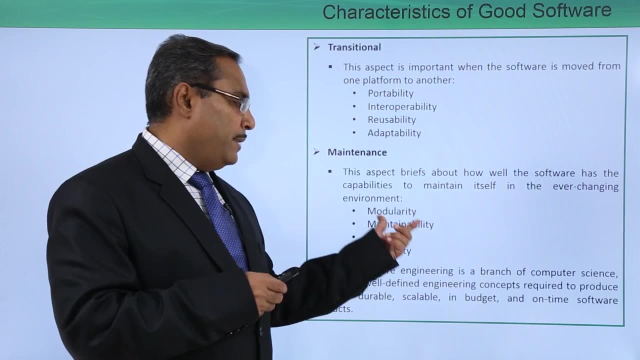 pre-existing version of the software. that will be also a good measure, whether the software is good or bad. So here, under this one, we are having four points, that is, the modularity, maintainability, flexibility and scalability. So these are the four points coming under this maintenance. 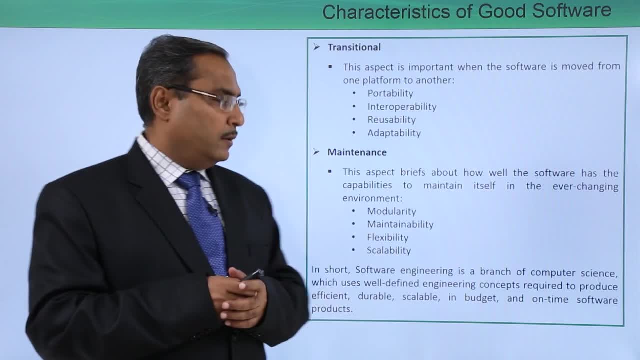 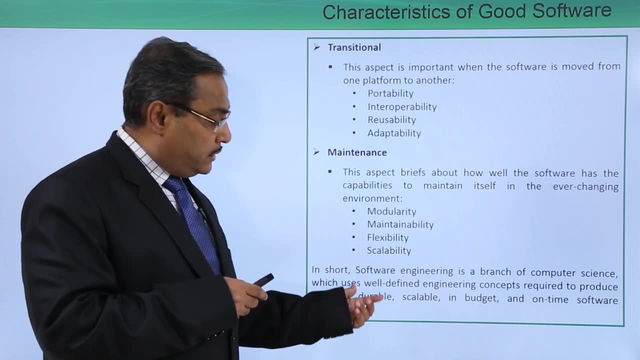 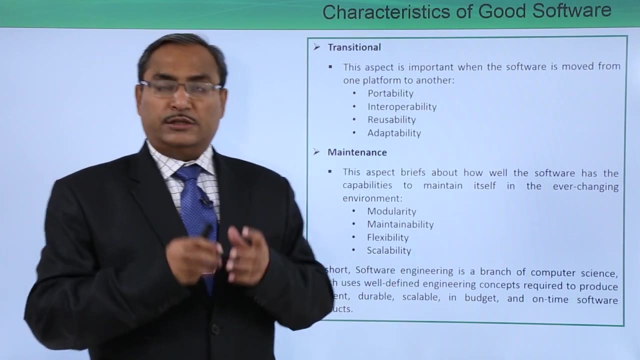 So, in short, software engineering is a branch of computer science which uses well-defined engineering concepts required to produce efficient, durable, scalable in budget and on time software products. So you should have the software with this respective features. that means it should be.